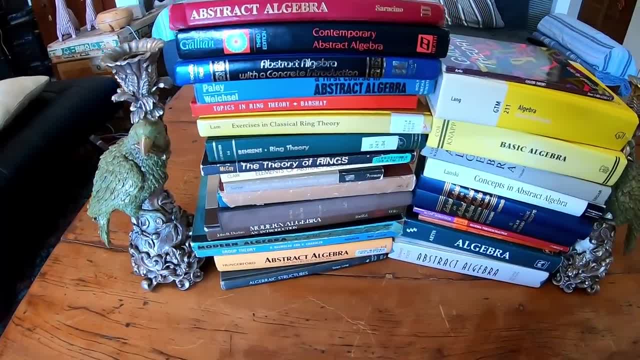 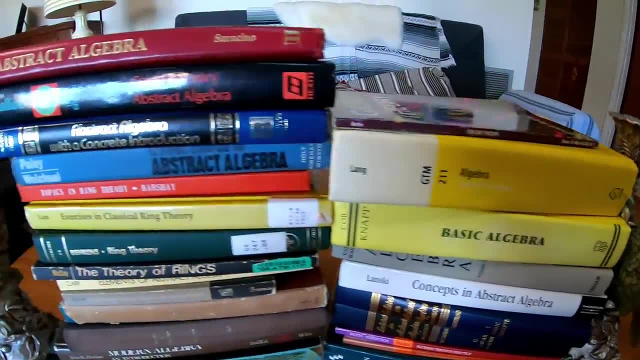 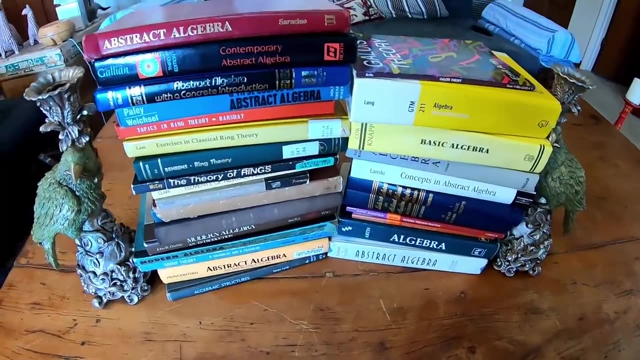 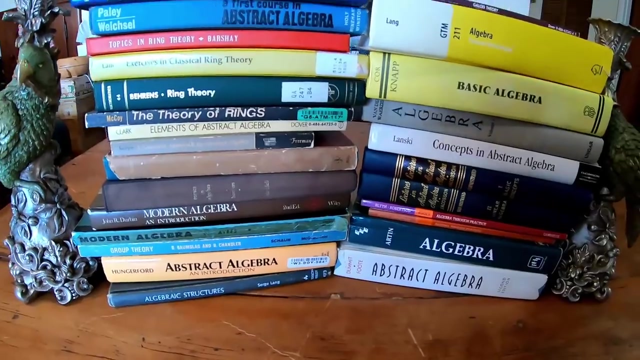 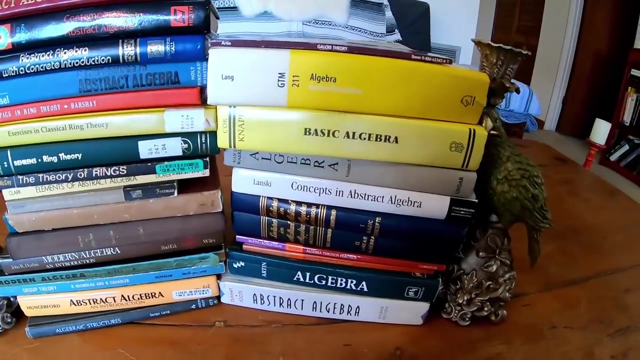 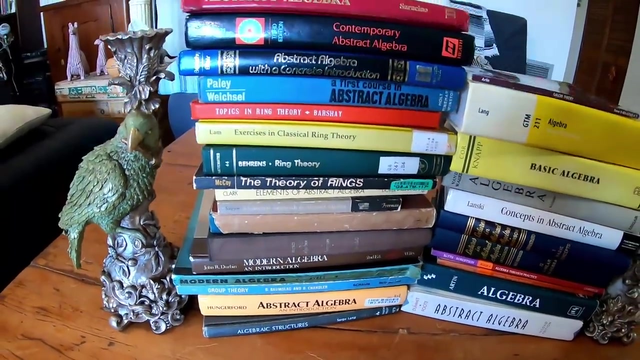 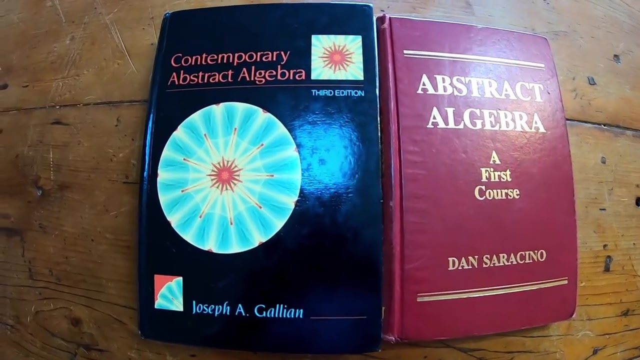 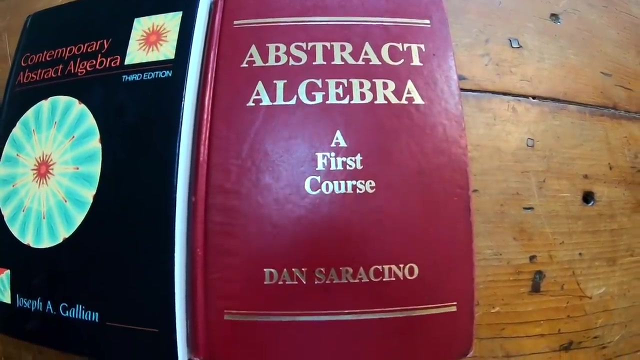 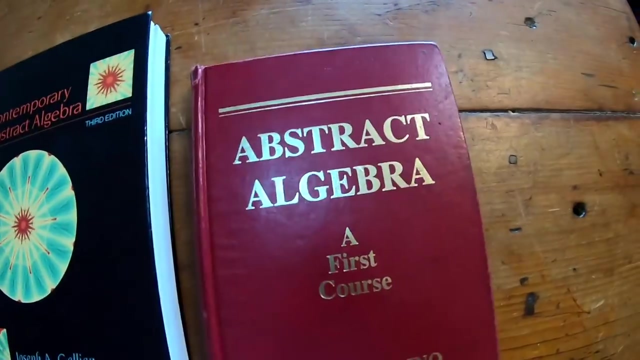 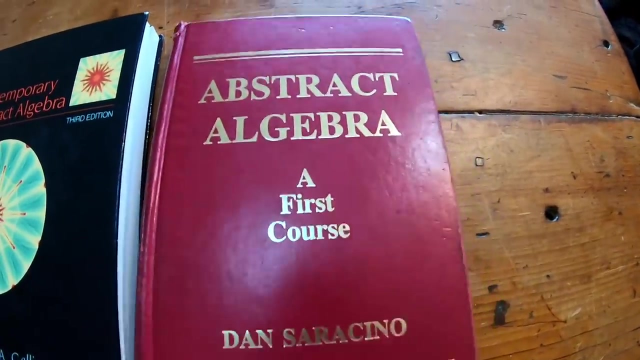 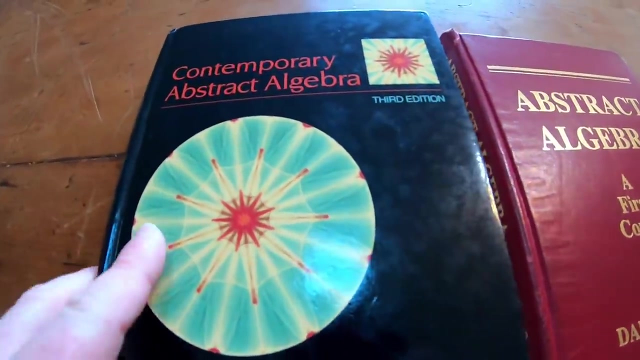 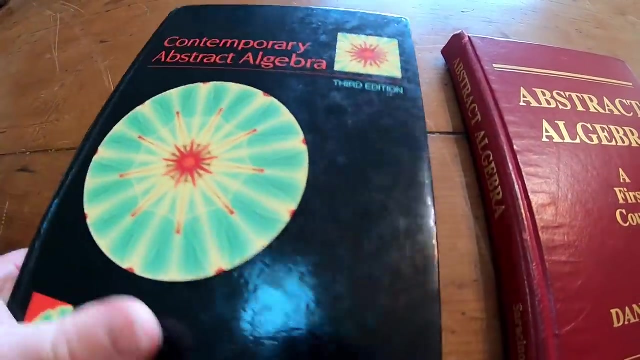 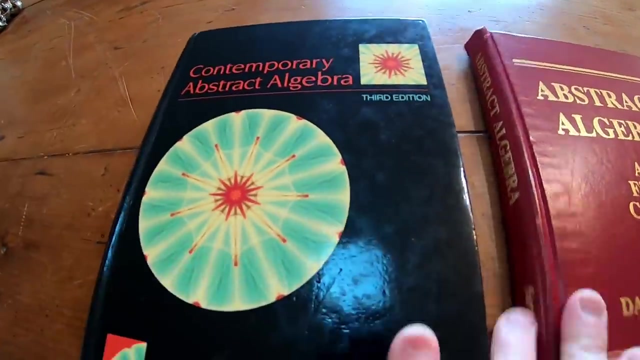 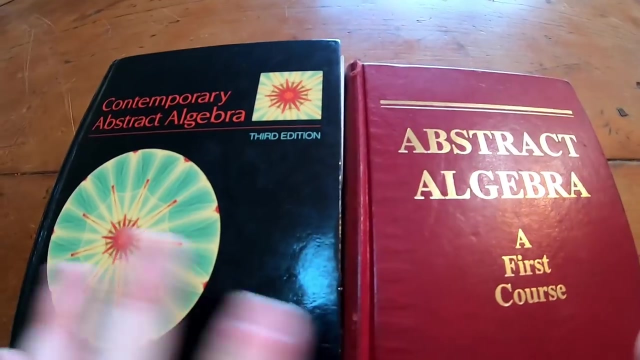 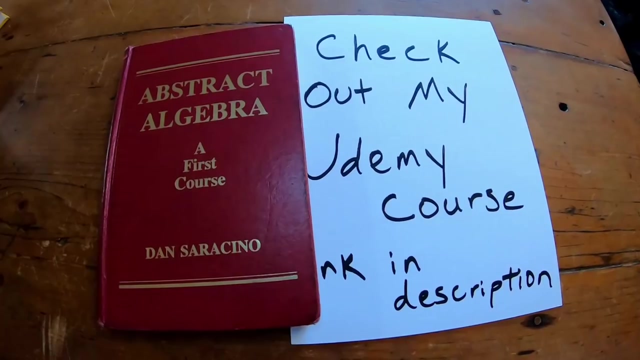 In this video, I'm going to show you how to start learning abstract algebra and progress through it in a somewhat linear fashion. We're going to talk about how to learn abstract algebra from start to finish. Now, by finish, I don't mean finish everything there is to know about abstract algebra. I'm not even sure if that's possible, but we will work our way up to definitely graduate-level abstract algebra. So a good starting point for abstract algebra is to try to use one of these books. This is my favorite book for beginners. This is Abstract Algebra, a first course by Dan Saracino. I have actually read this entire book, and I've done almost every single problem from this little book. The only downside of this book is that it doesn't have more information. So you can get this book for just a few dollars if you do some research online, try to get a used copy. And this one is a little bit more advanced, but it's still a beginner book. This is Contemporary Abstract Algebra by Joseph Galleon. A good friend of mine from New Zealand told me about this book many, many years ago, and he used this book for a course he took, and he liked it a lot. And I think that this book has good examples. So always think of the Galleon book as a book of examples. So both of these books can be purchased fairly inexpensively and are really, really good starting points for abstract algebra. So I do have an 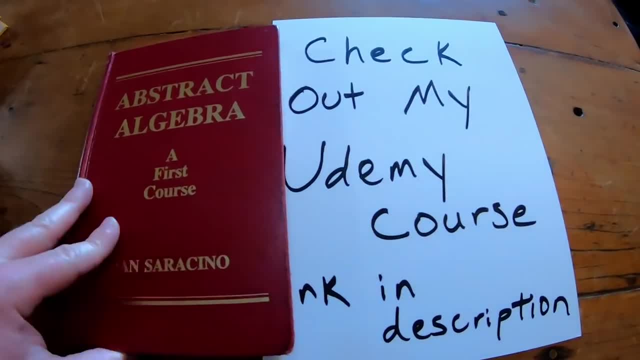 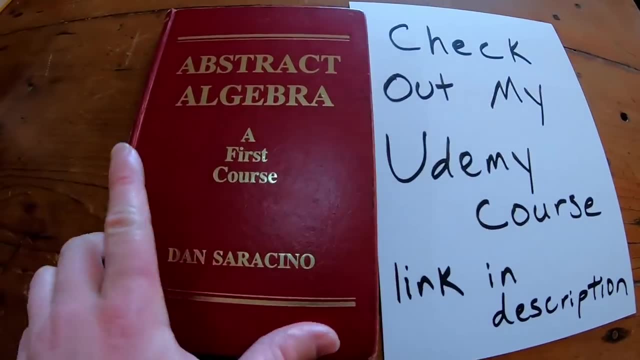 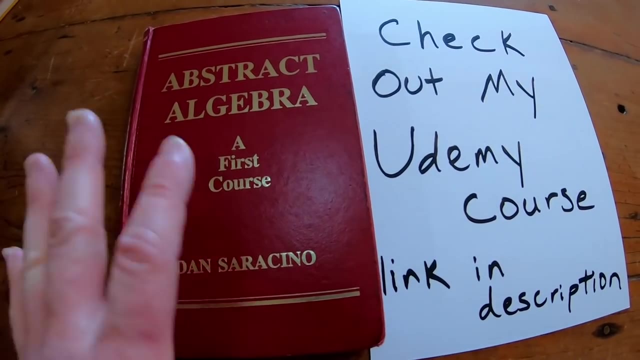 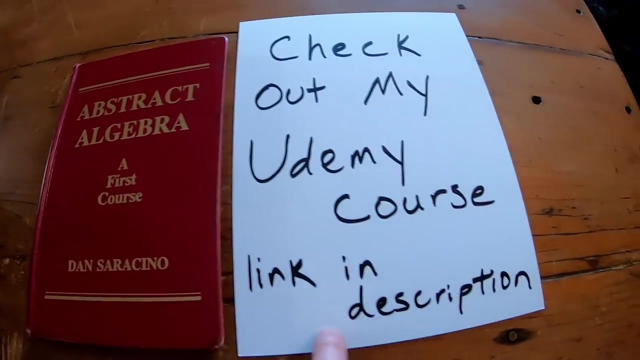 abstract algebra course on Udemy, which is really good for beginners, and the link is in the description. And the reason I put this book here in the video so you can see it is because I feel that if you're going to get the course, I think this might be the best book to get that goes the along with it. So the course is created from notes that I made from this book and from lectures and from other books, but mainly it kind of follows the order of this book. So if you get this book and you get the course, that'll go well together. So I just wanted to mention that just to make sure 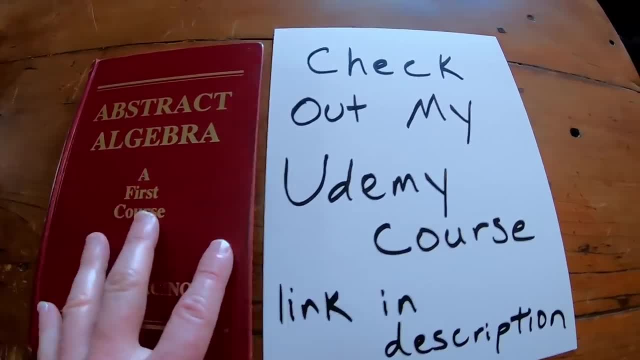 that if you do get the course, I think this book will help you. How much math do you need for this? 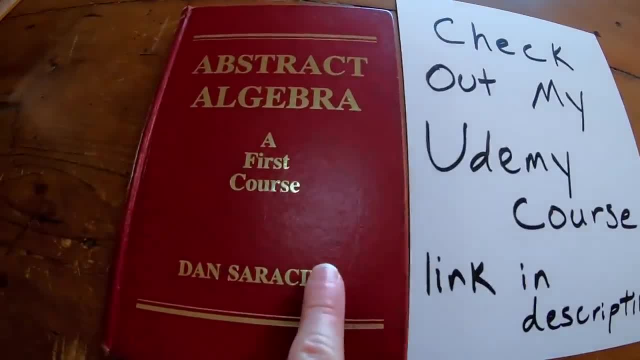 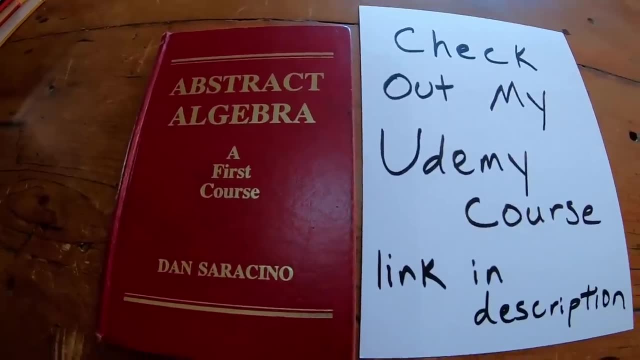 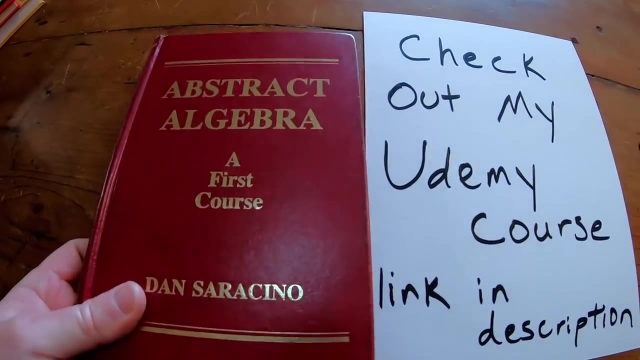 You should know how to write proofs, honestly. Like a prereq for this course in college is like and a bunch of other math classes. They make you take Calc 1, Calc 2, Calc 3, DE, proof writing, linear algebra, then you can take abstract. So it's a 4,000 level course in the U.S., right? This is an 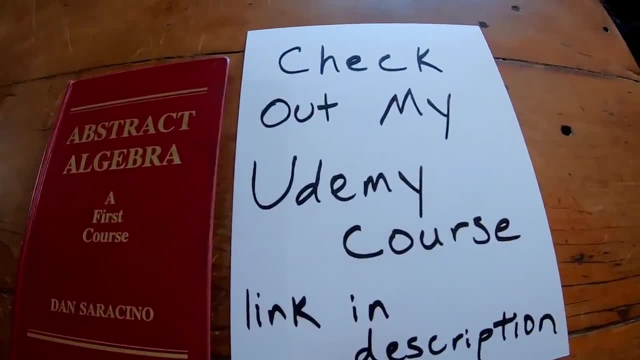 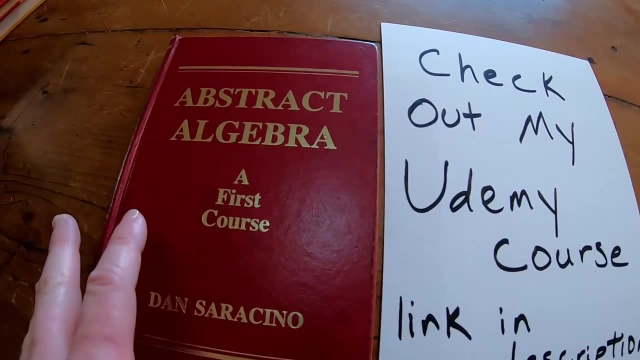 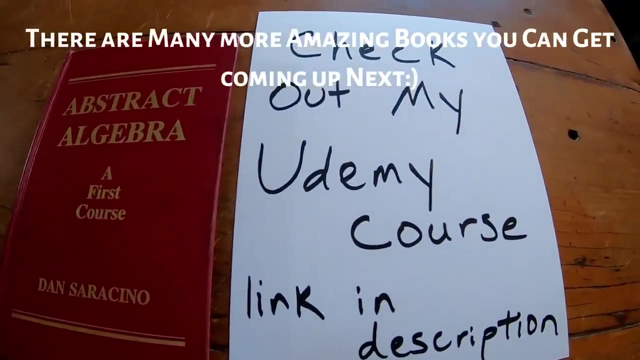 advanced course, but you could jump into it, I feel, because of the way it's structured. Like it starts with binary operations. I tried to follow the model in this book so that you can actually learn the stuff and just jump into it and learn what a group is, you know, learn how to show a set as a group, you know. 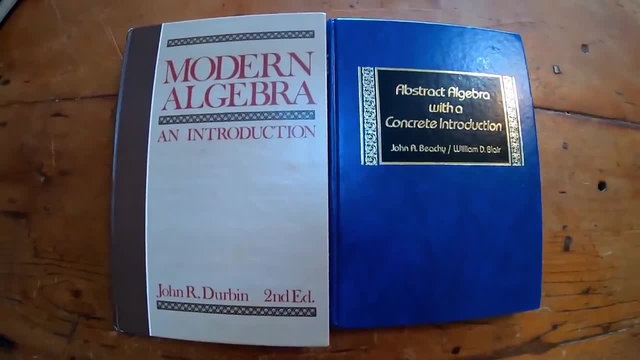 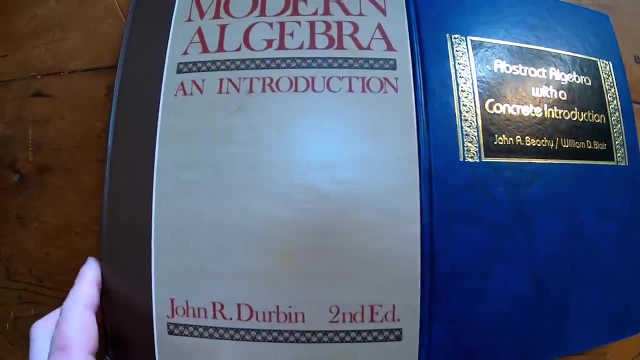 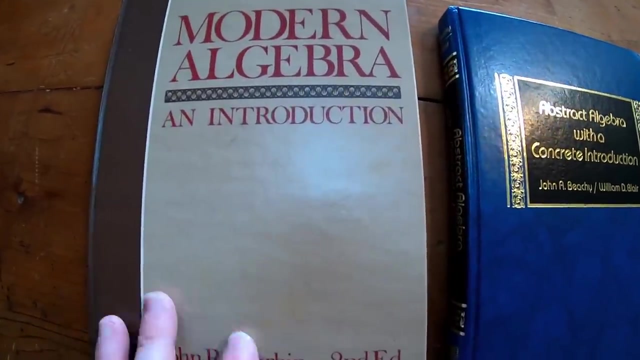 Learn some really cool math. Here are two more beginner level books, but they're a little bit more advanced, perhaps. Modern Algebra by Durbin is an introductory book, and it's written very, very well. And it does contain some like specialized topics that you won't find in other books. So this is also a good beginner choice if you're trying to learn abstract algebra. 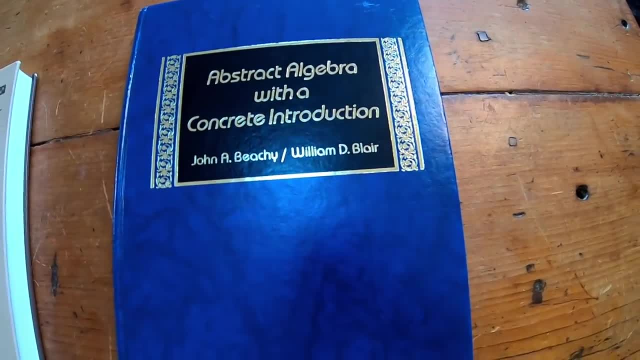 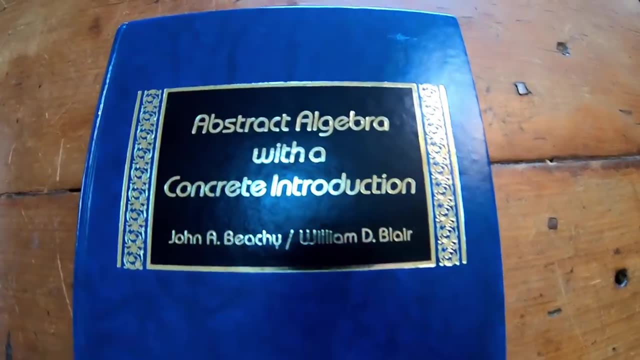 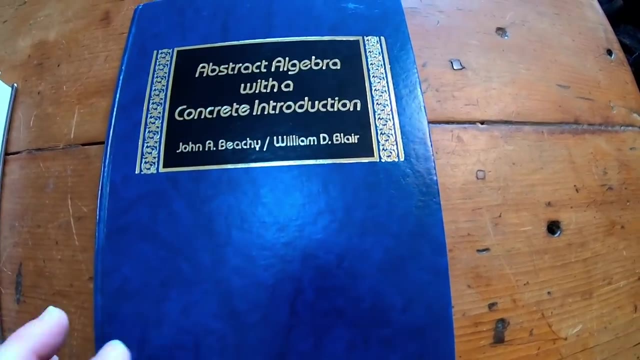 And then this one here is extremely well written. And again, it's a beginner book, but it talks about the importance of learning abstract algebra. So if you're trying to learn abstract algebra, it talks a little bit more about fields. In fact, this is the book that I used to teach myself field theory. So out of all of the books you saw at the beginning of this video, this is the one that, in my opinion, explains it in the most beginner-friendly way. 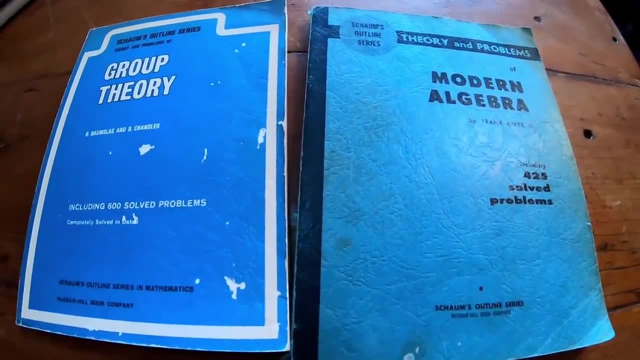 No abstract algebra video is complete without mentioning the Shams series of books. So this is the one on group theory, and this is the one on modern algebra. Both of these are pretty good. 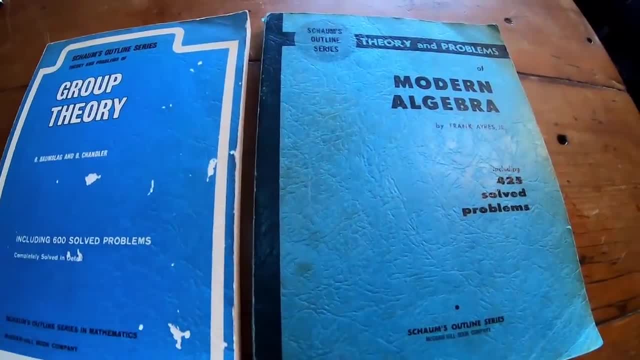 So if you have extra money, I would say get them. But the other books I think in this video are good enough to where you don't actually need the Shams. So I've had these for a long time, and honestly, 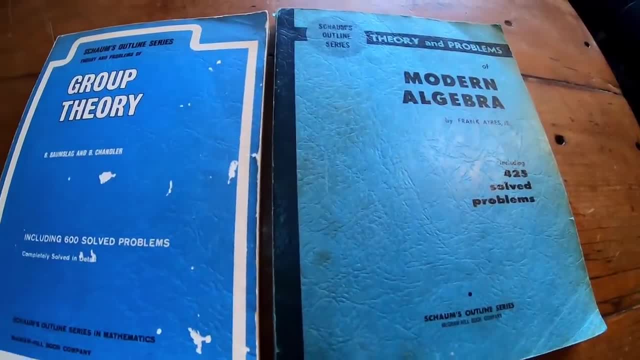 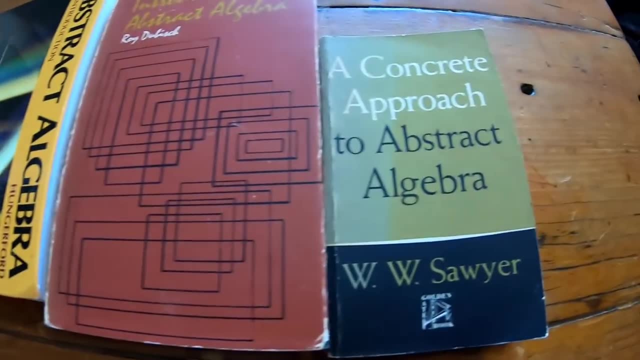 I haven't had to use them that much because I feel like the other abstract algebra books are really just enough. Here we have three more beginner books. So the one on the right, 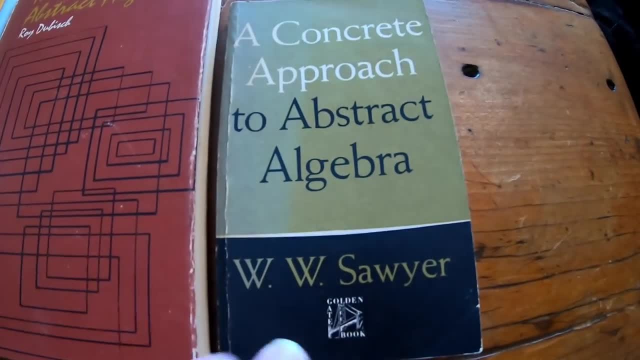 A Concrete Approach to Abstract Algebra, this was given to me as a gift. This one is quite readable, but it's very, very beginner. It's almost, 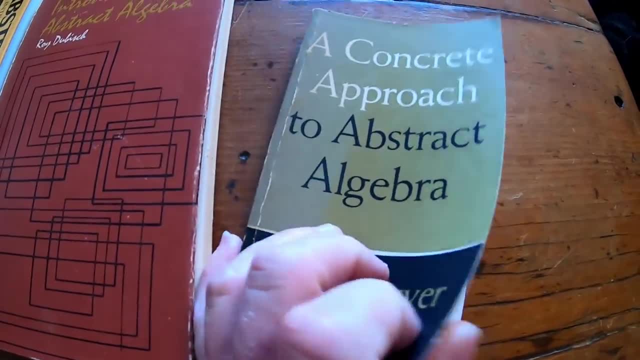 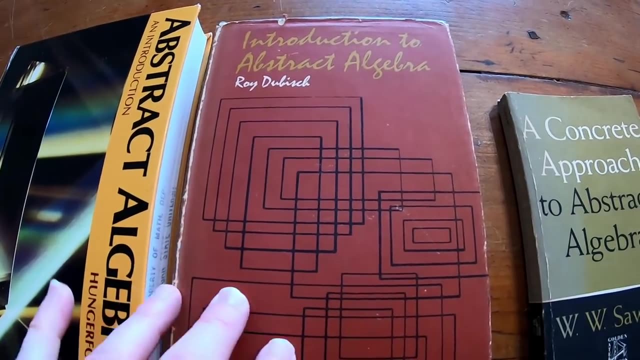 too beginner. So if you can get it really inexpensively, I would say get it. Otherwise, I'd say maybe skip it. This one, An Introduction to Abstract Algebra by Roy DeBitch, is also quite beginner-friendly, and it was also a gift. And out of all three of these that you see here, 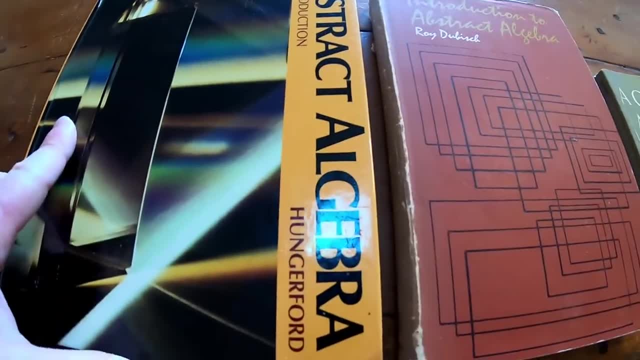 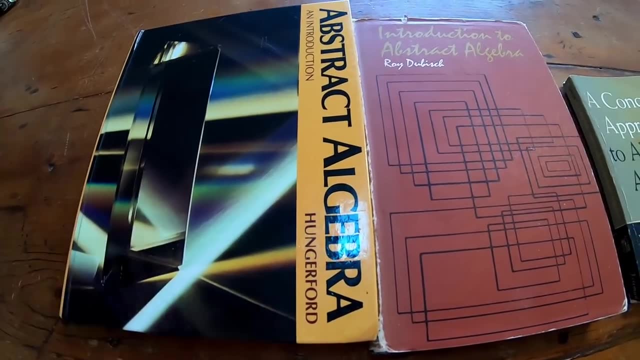 I think this is the best one. This is Abstract Algebra by Hungerford. Now, Hungerford has a couple books on abstract algebra. In particular, he has a graduate-level book, which is awesome, which I have, but I can't find it. 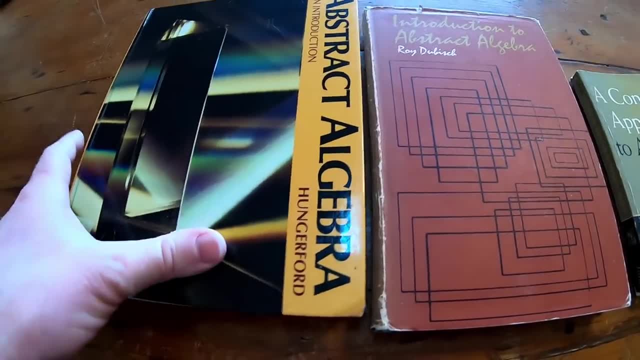 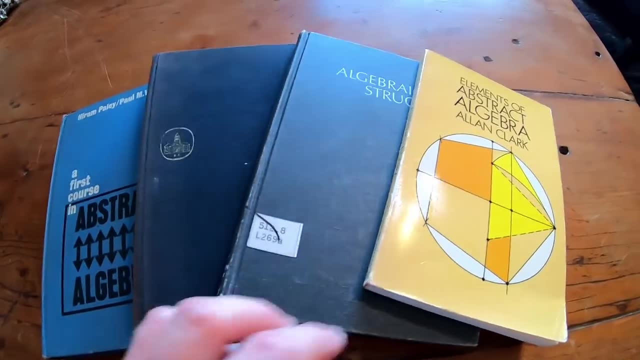 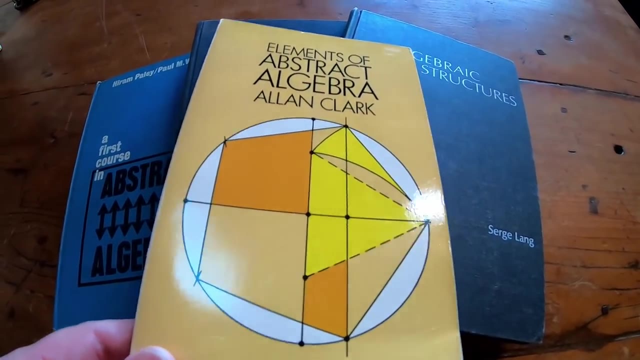 But I have a graduate book, and it's extremely good, and it's very, very beginner-friendly. Here we have what I like to consider our middle-of-the-road books. So the first one here, Elements of Abstract Algebra by Alan Clark, is one that was recommended to me by this guy I used to talk to in a math chat room years ago. And I bought this book because he said it was awesome, 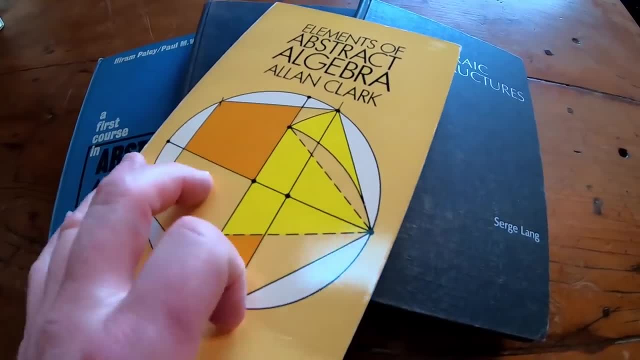 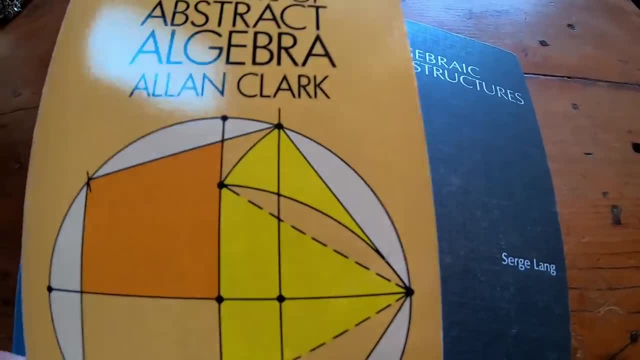 Recently, someone left a comment saying that they taught themselves abstract algebra with this book, 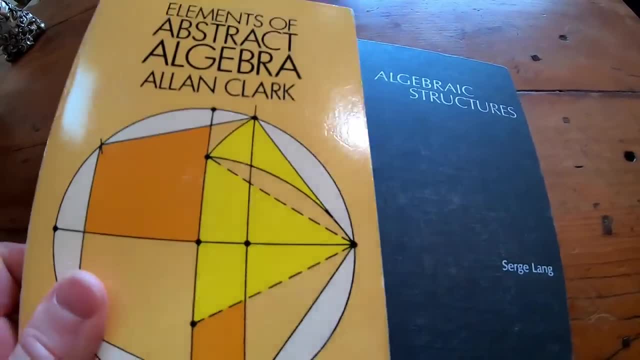 and I was like, wow. If this is the only book you use to teach yourself abstract algebra, you know, props to you. It's a pretty tough one. So again, if you have the extra money, 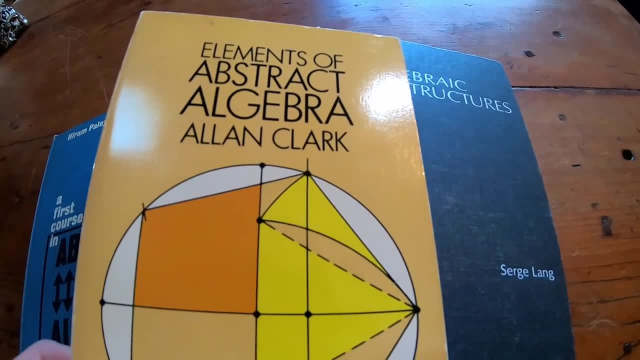 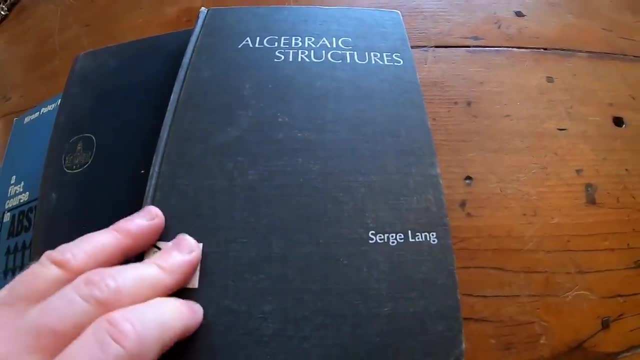 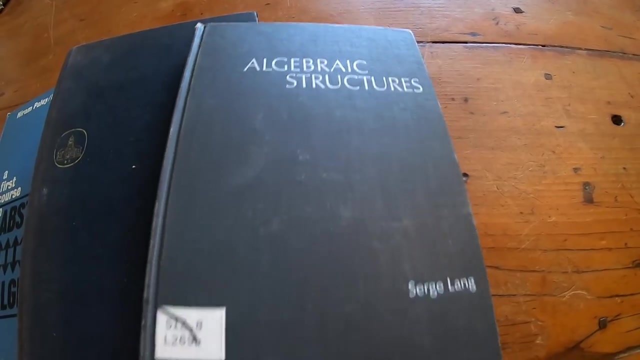 it's a Dover book. It's not that expensive. It's Elements of Abstract Algebra by Alan Clark. This one's a really good one, Algebraic Structures by Serge Lang. This is basically Lang's undergraduate book on abstract algebra. It talks about all kinds of topics, it's got groups, rings, fields, modules, vector spaces. Really, really good choice for beginners. 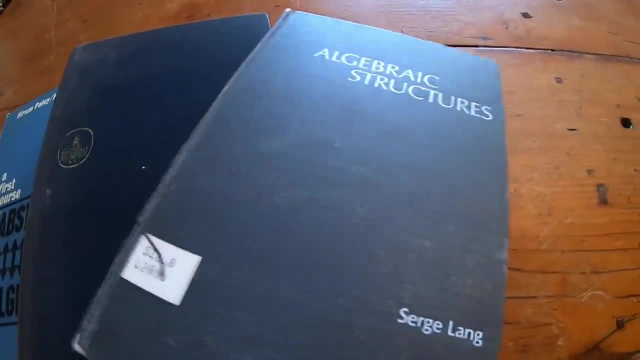 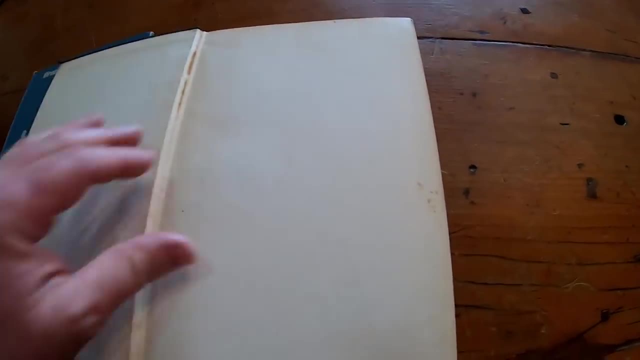 I put it in the middle of the road list, though, because it does have some more advanced topics. This is a famous one. This is Topics in Algebra by the famous Herstein at a friend in grad school 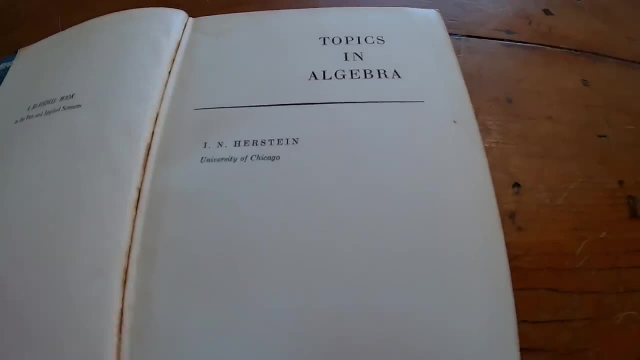 who pretty much worshipped this book. This is extremely well written. I feel like this is a must-have for anyone learning abstract algebra. Again, a middle-of-the-road type of book. 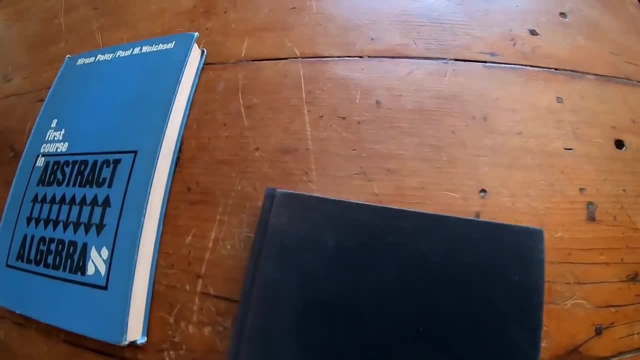 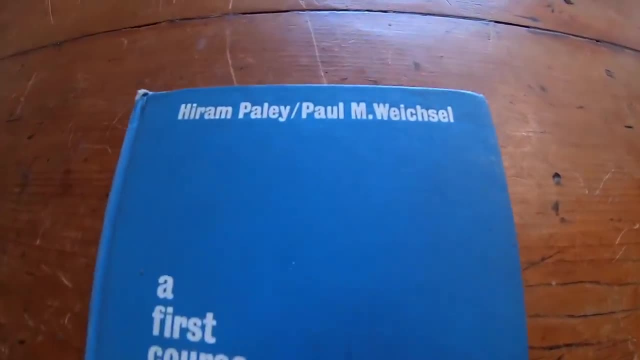 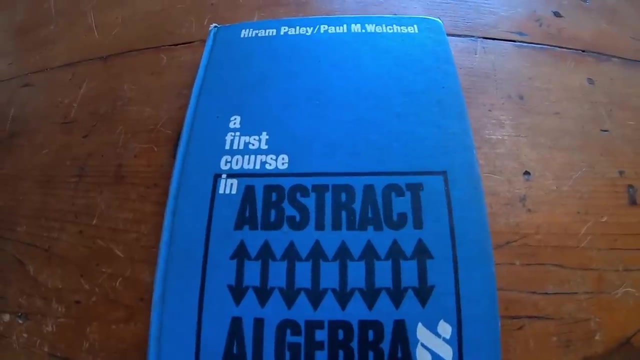 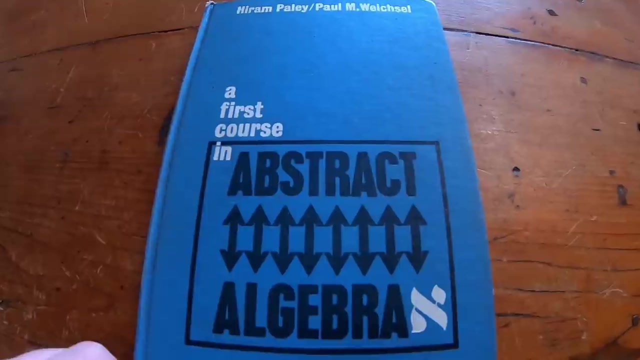 Supposed to be for beginners but it's a little more advanced. And here is one that you've probably never heard of which I really like. It's a First Course in Abstract Algebra by Pillay and Weishull. And I don't think this book is still in print. I'll try to find links on Amazon so you can read the reviews for these books. This one's really good. It's got some downsides. Some of the notation is a little bit weird, the function notation. But otherwise, this is a fantastic book. 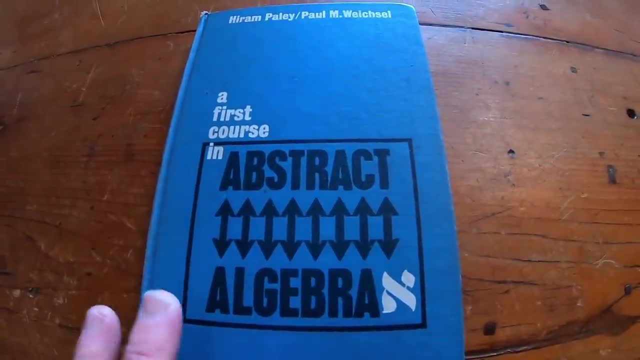 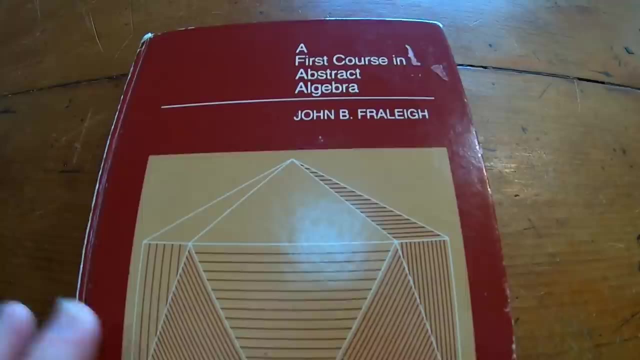 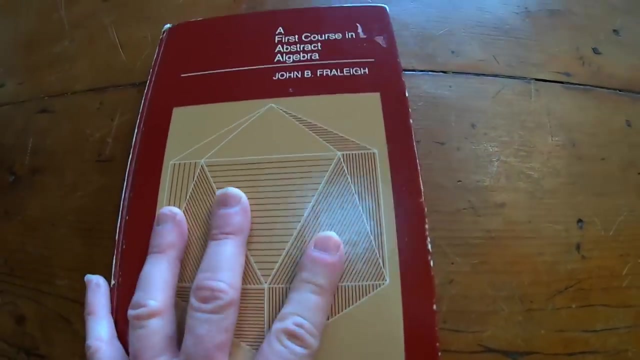 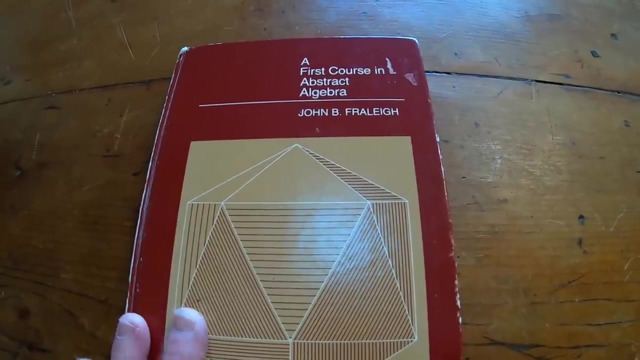 And it's intermediate level. This has more advanced stuff in it. So I had to talk about this book separately from the other books because this book is really good. This is a beginner slash intermediate level book. It's kind of like an advanced beginner book. It's the one by Fillet. And this book was recommended to me by my abstract algebra professor when I was an undergrad. And it's extremely well written. 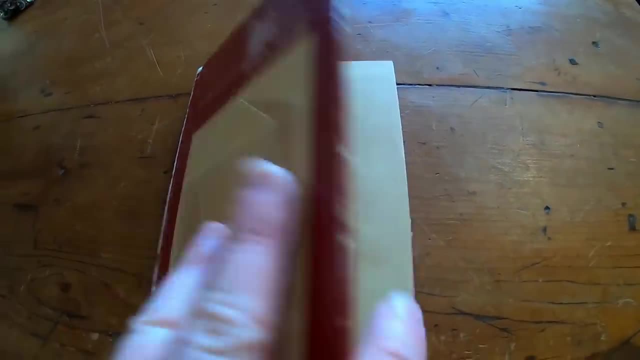 It just reads really, really well. There are some downsides to it. Some of the notation is a little bit... 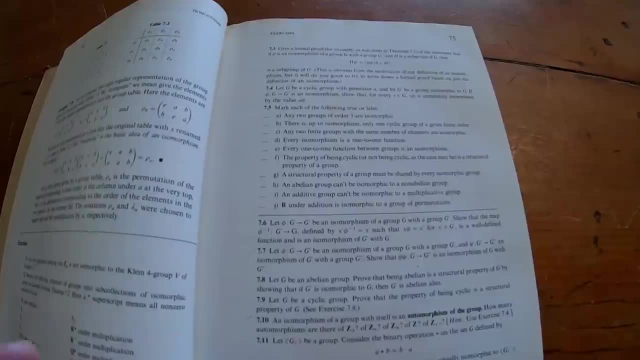 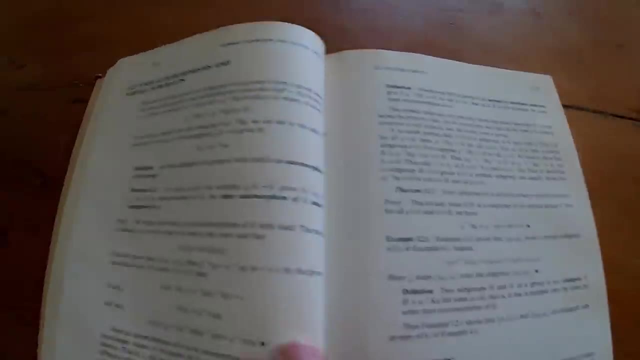 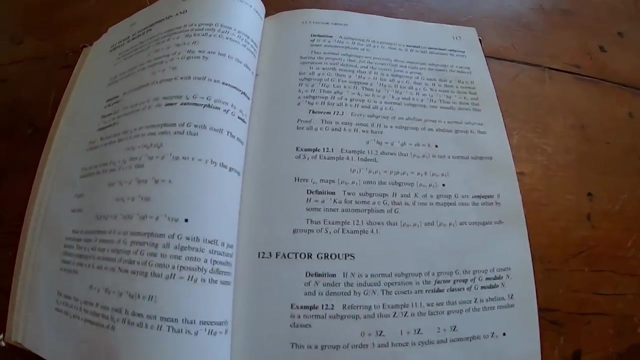 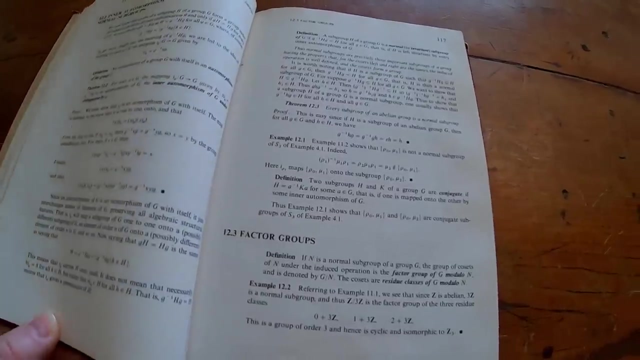 different. For example, Fillet does his cycle multiplication backwards from other books. But otherwise, this is a really good book. It's got really small sections. You see 12.2 is just one page and a little bit more. Then you go to 12.3. So it's like small, digestible pieces of information. This has way more information than, for example, the Saraceno book, which I mentioned at the beginning of the video. So definitely a good beginner choice. If you can get this book 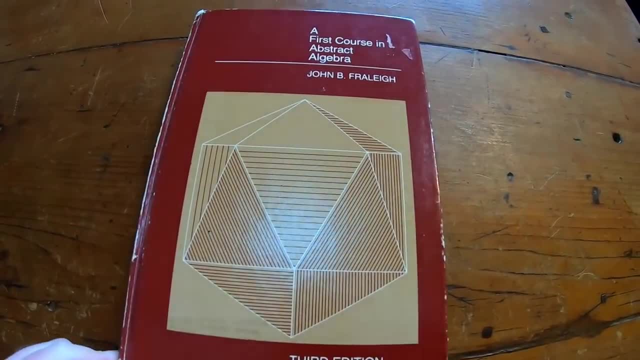 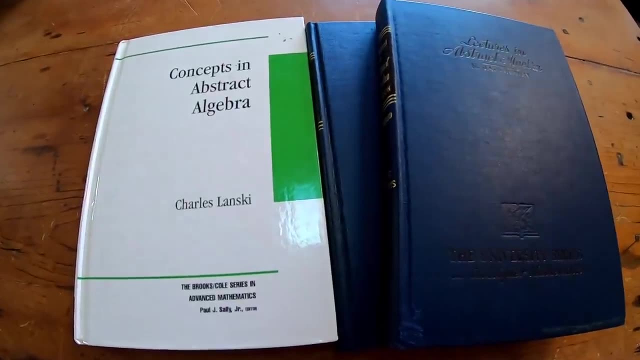 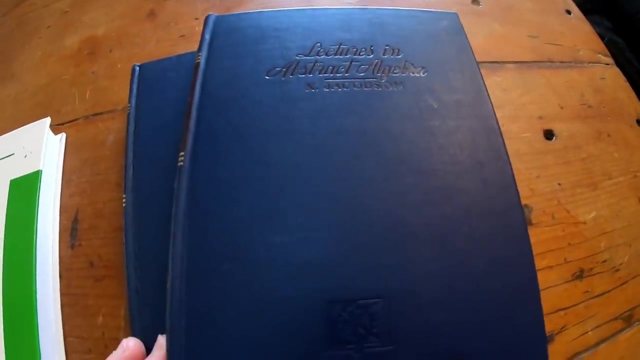 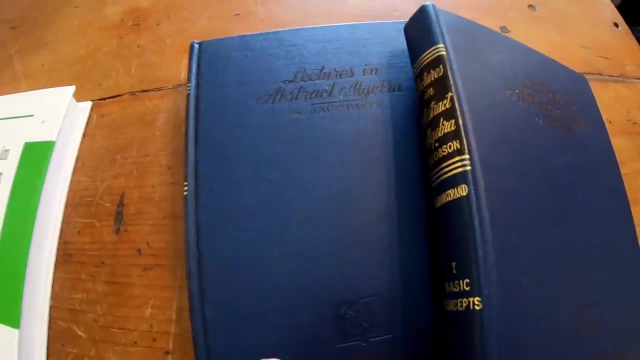 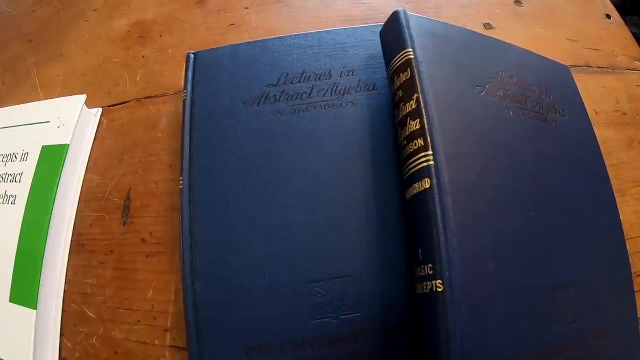 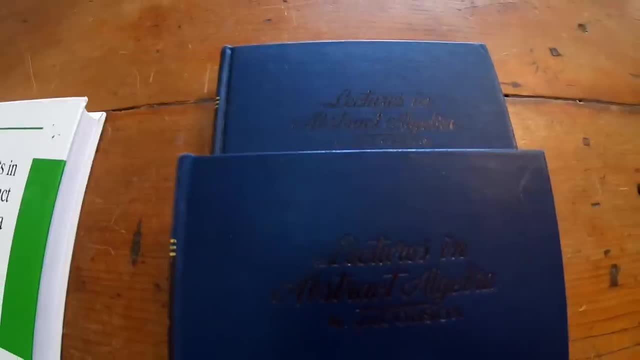 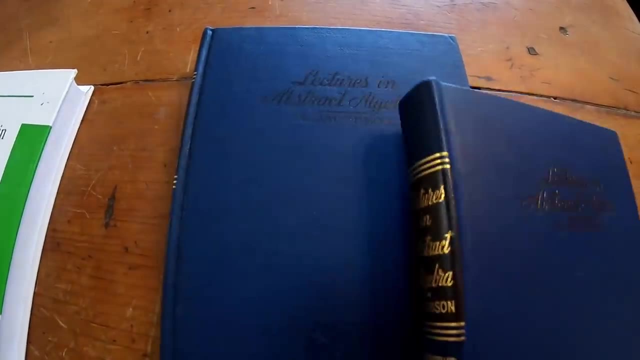 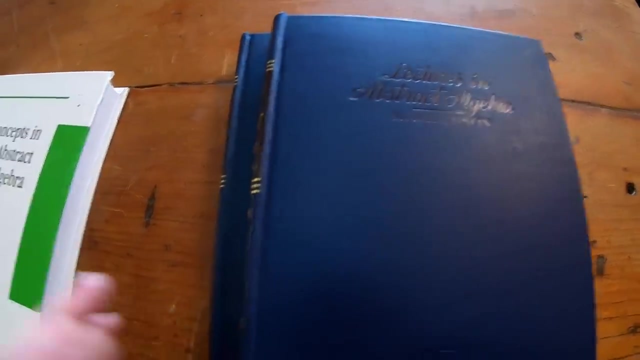 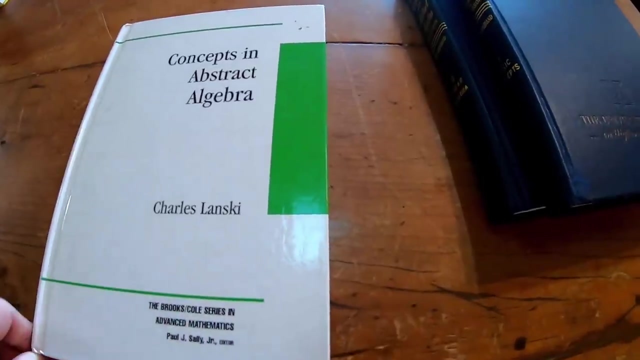 a good book. It's a good book. 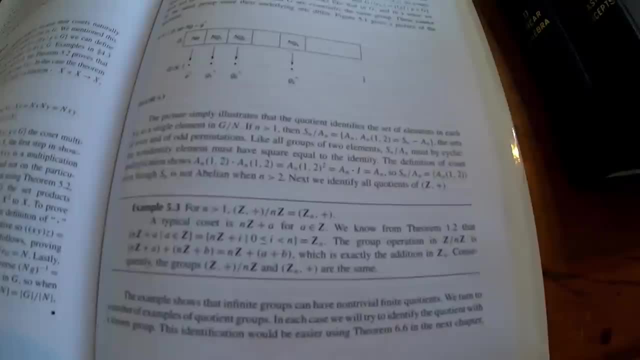 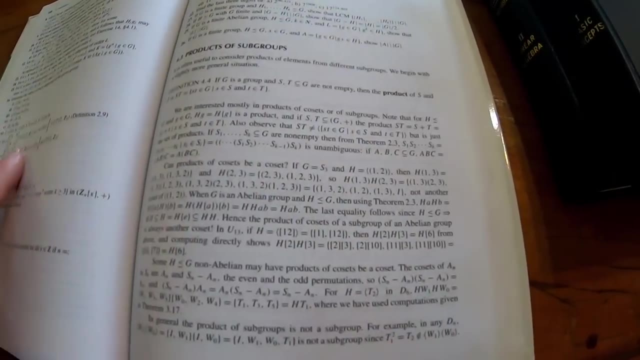 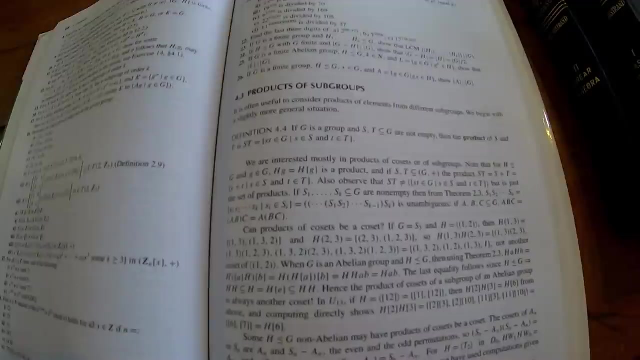 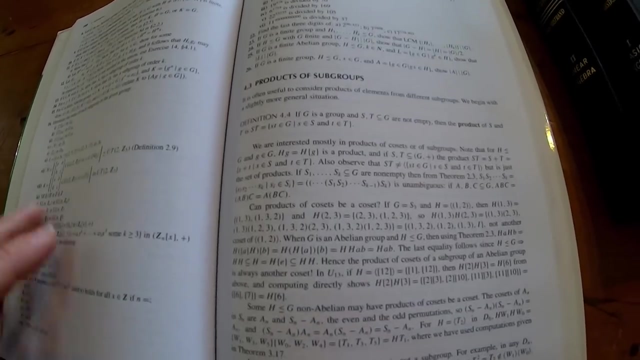 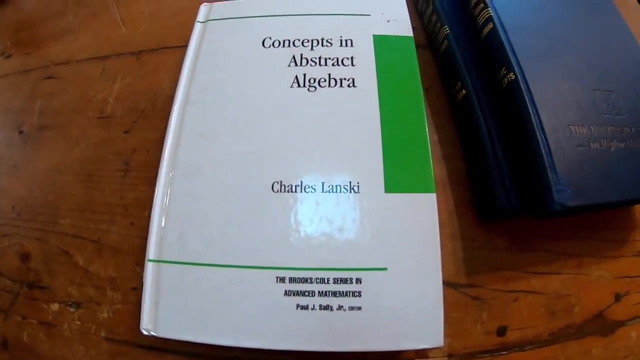 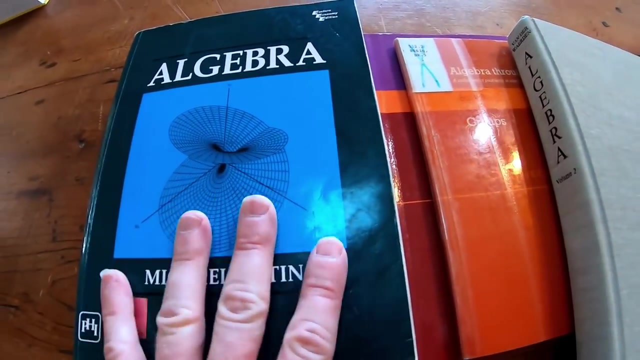 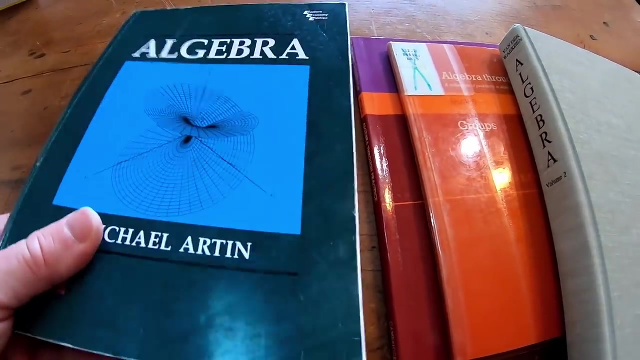 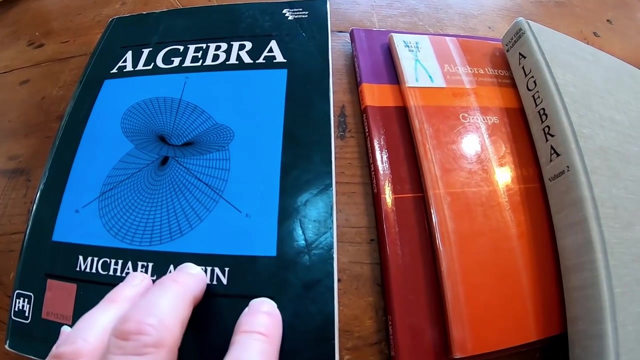 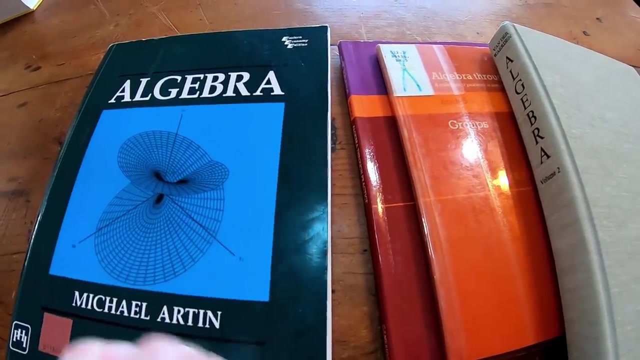 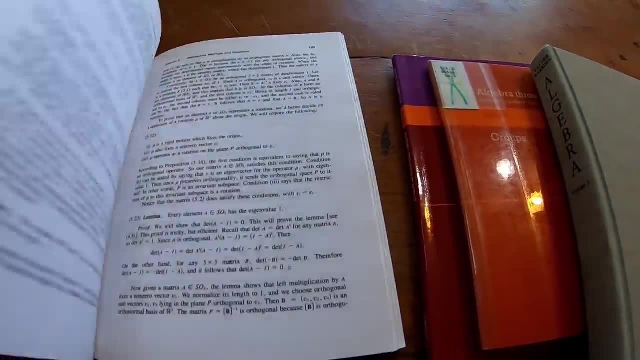 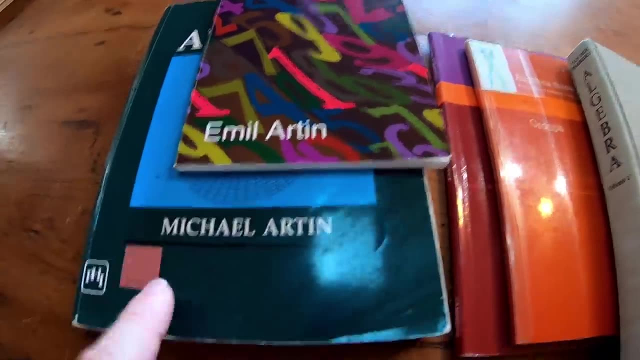 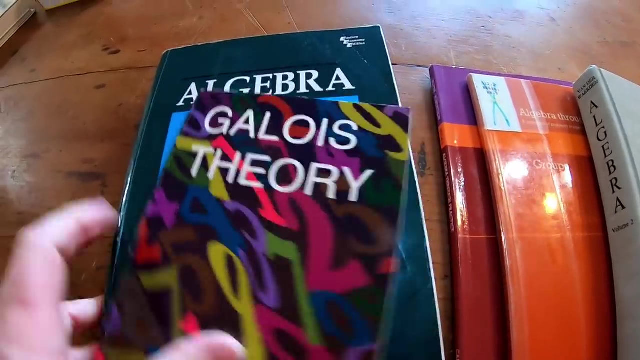 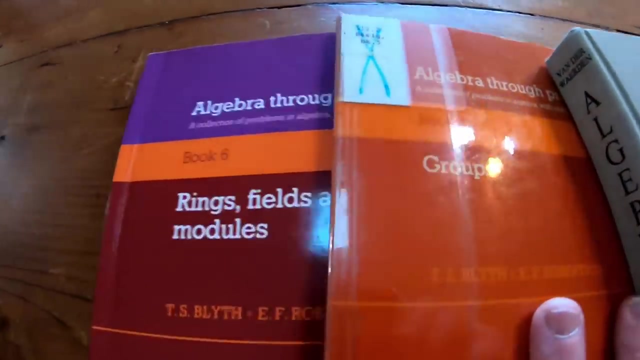 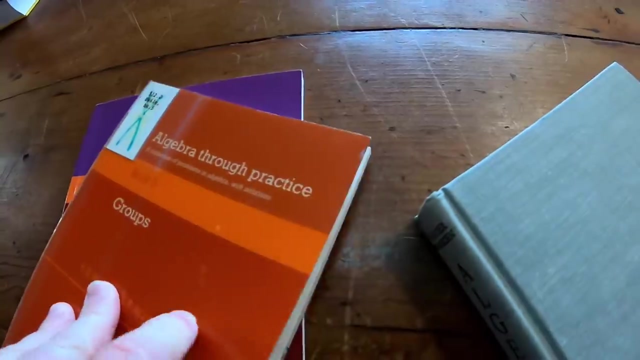 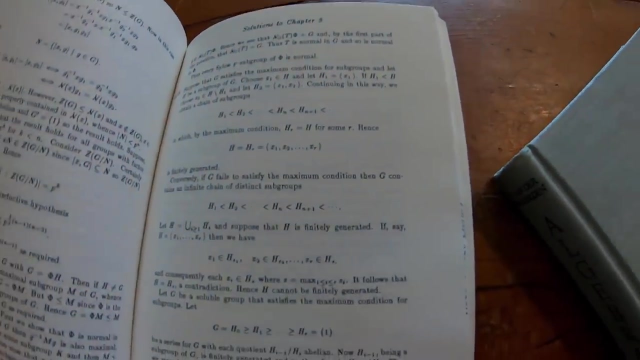 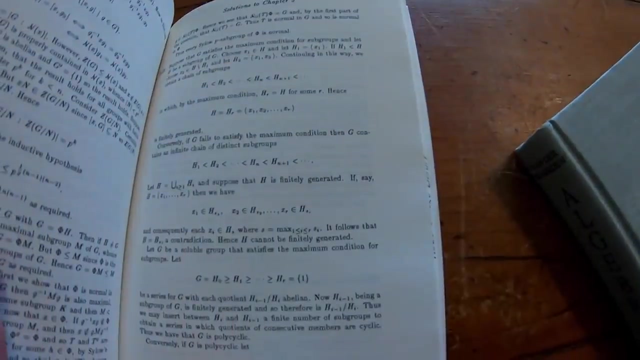 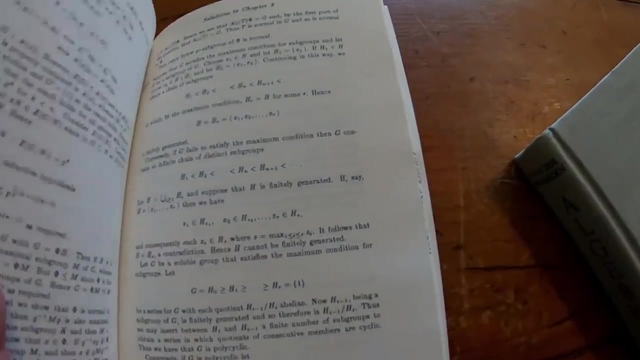 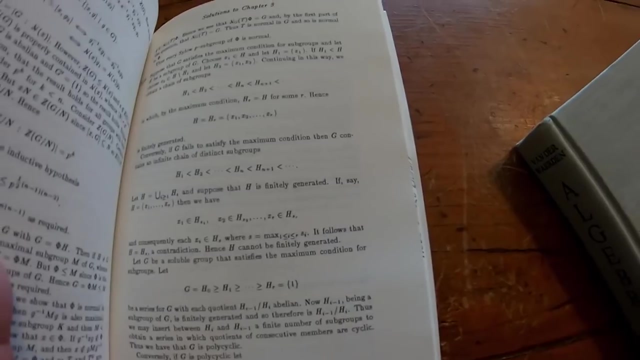 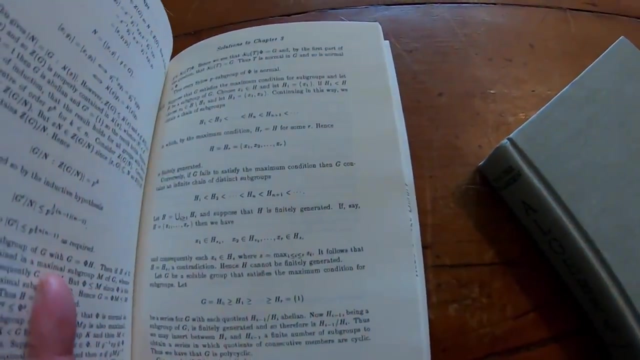 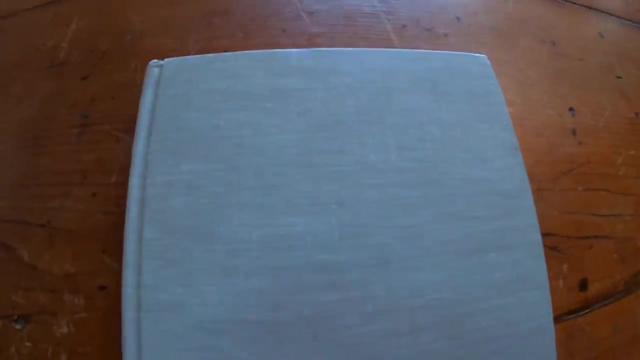 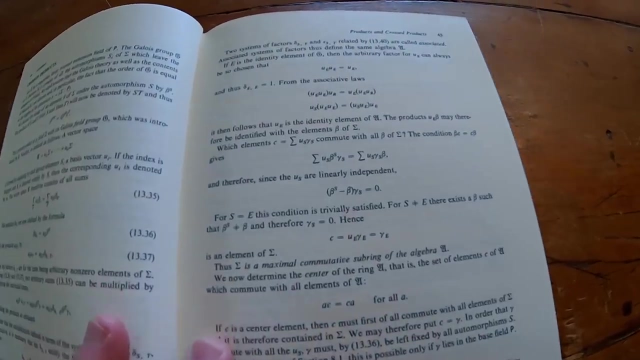 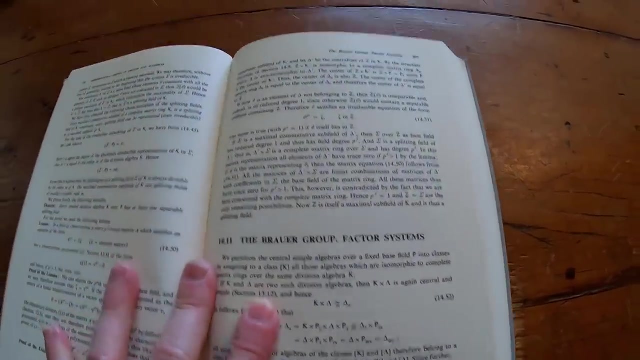 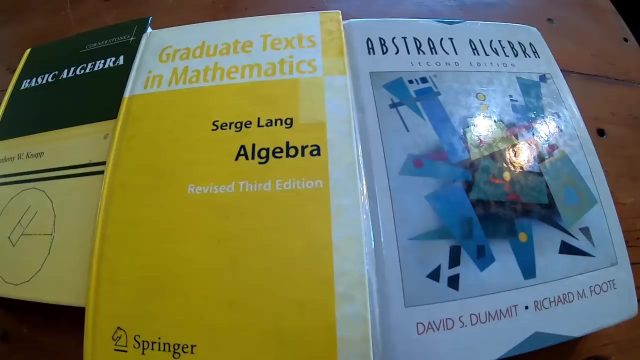 And this is a great book. His father was Emil Artin, which also wrote a fantastic book. Here, let me just grab it. Here it is. It's Galois Theory. So this is the father and this is the son. And this is also an advanced book, but again, you could probably read it and understand some of it. Both of these books are very well written by both of the Artins. Classic books. These here are part of a series called Algebra Through Practice. This is the one on rings, fields, and modules, and this is the one on groups. And these are problem books. These books have full solutions. Let me just open it so you can see. These books have problems and full solutions to proofs and exercises in groups and in rings, fields, and modules. And I put these in the advanced section because the problems are hard. These are not beginner books, so don't think that you can buy these books if you're new to abstract algebra and learn abstract algebra. The problems are a little bit more advanced. Even though you have solutions, it's still pretty hardcore. If you can find these books inexpensively, I highly recommend getting them. They're kind of expensive, I think. These are kind of hard to get and they're kind of pricey. This one I wanted to include here because I couldn't find another place to include it. It is advanced, but it's a good book. But it's not like the most advanced. This is the classic by Vander Warden. This is Algebra. There's multiple volumes. I just included volume two in this video. This is a classic old school text on abstract algebra, and it is considered quite, quite advanced. All right, here we have three seriously thick, hardcore, advanced abstract algebra books. So Basic Algebra is a graduate level book. I used this for a course in grad school. I'll be honest, when I took the course, I already knew that this was going to be a good book. 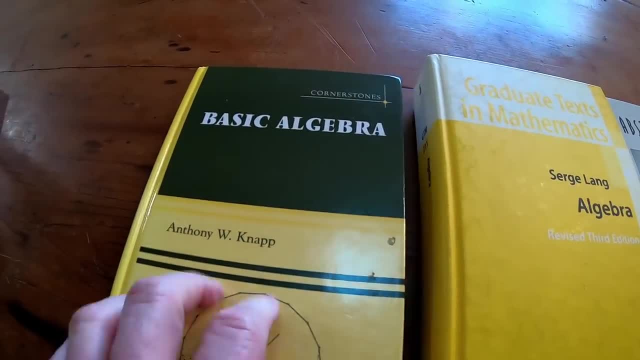 I knew a lot of abstract algebra, including graduate level, so I didn't have to use the book too much. We had some homework from it. I felt the explanations were pretty good. 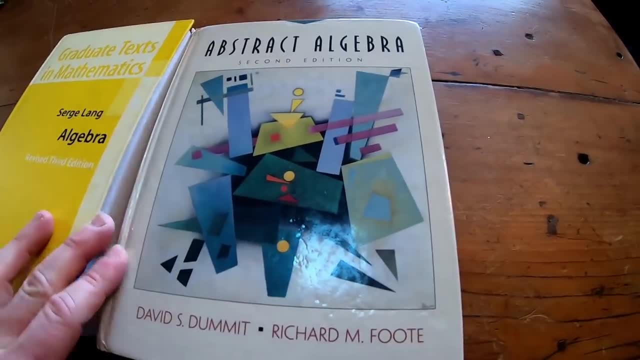 This one here, Dumb It and Foot, is a must-have for anyone serious about abstract algebra. Some people might consider this a beginner book. That's fine. I think it's grad level for sure. 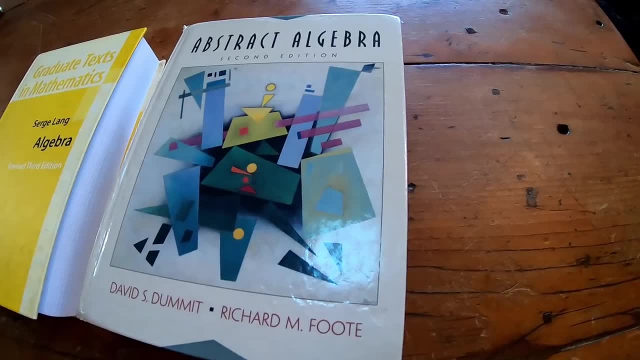 It has a lot of topics. It's a great reference. If you have to get one advanced book, I say maybe get this one because it serves as a great reference and it has a lot of information. 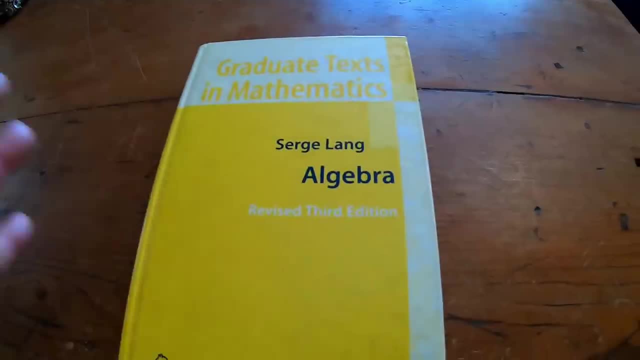 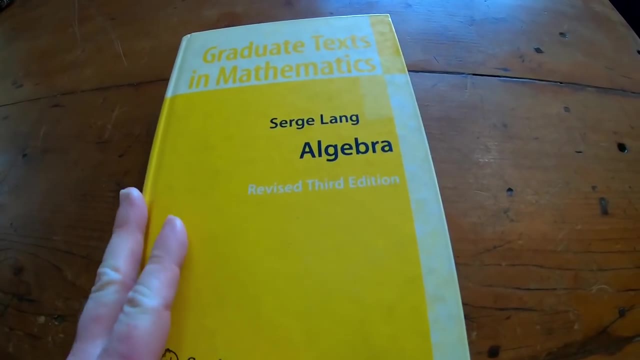 Then at the end, we have what many people consider to be the Bible of abstract algebra. It's Lange's Algebra. This book has some serious math. My copy is brand new. I bought it brand new because I felt that I wanted to get a new copy. You know, I wanted my copy to be new. 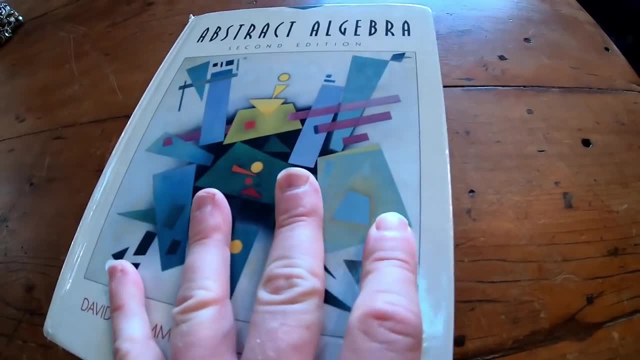 I got my copy of Dumb It and Foot, by the way, used, and some of the pages come out. So that's one of the disadvantages of trying to be cheap and getting cheap books. 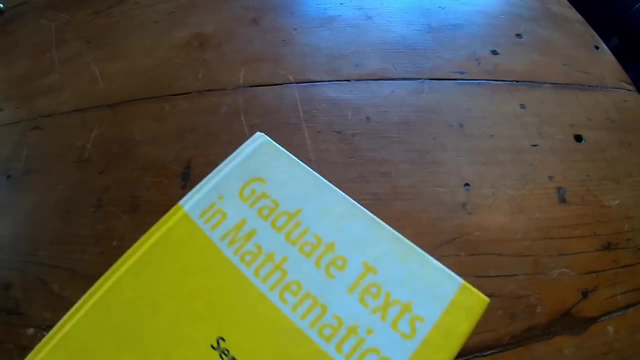 But this one, if you're serious about algebra, this is a must-have. But this one, if you're serious about algebra, this is a must-have. This is a classic. 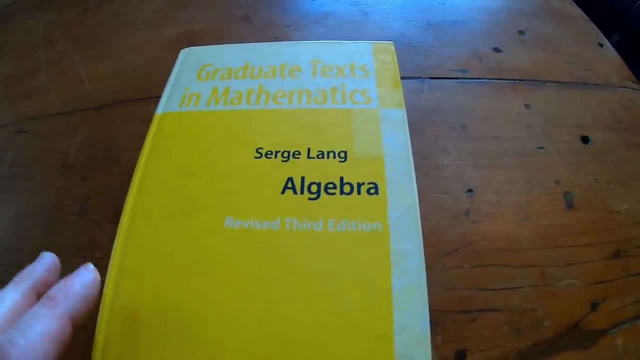 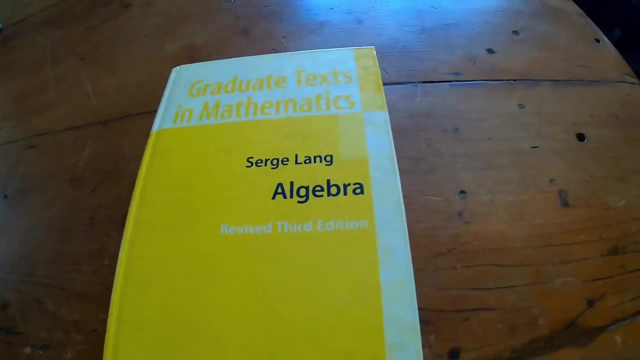 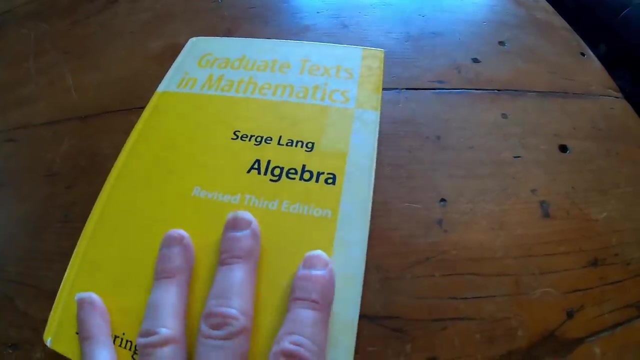 A lot of people talk really badly about this book. They say you can't learn from this book. I feel like when I was in graduate school, I used this book a lot. I referenced it a lot. It had a lot of good information on, for example, semi-direct products. I found more information in this book and in Dumb It on semi-direct products than in the other books I had. So it's a good reference. It's a good book. 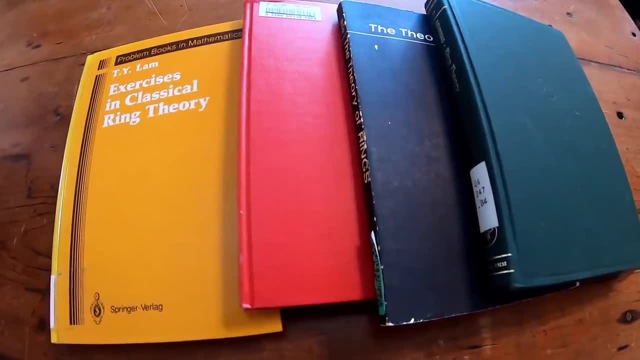 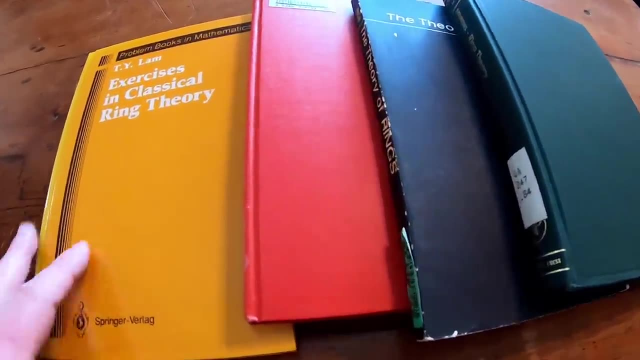 So here we have four books on ring theory. That's right. So algebra, it doesn't really finish. go forever. So there's a whole subject called ring theory. It's a study of rings. This is a 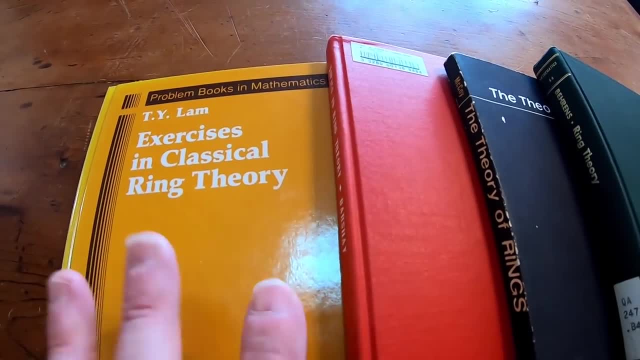 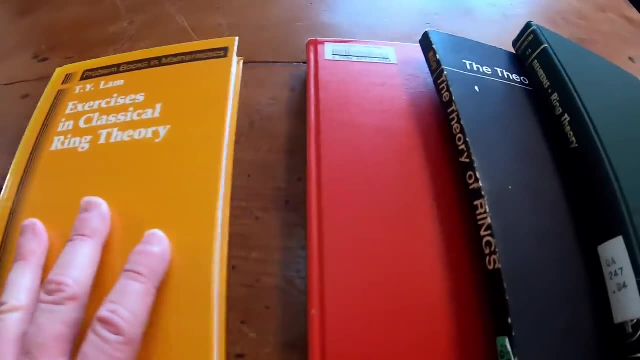 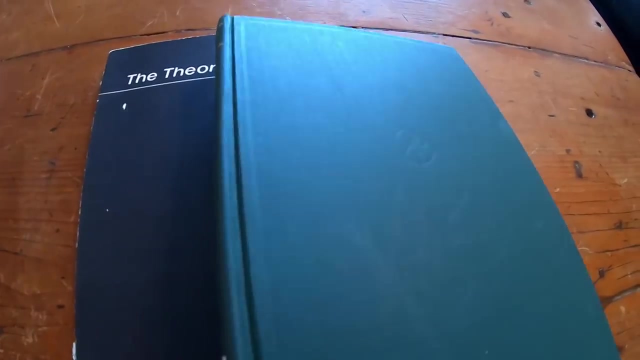 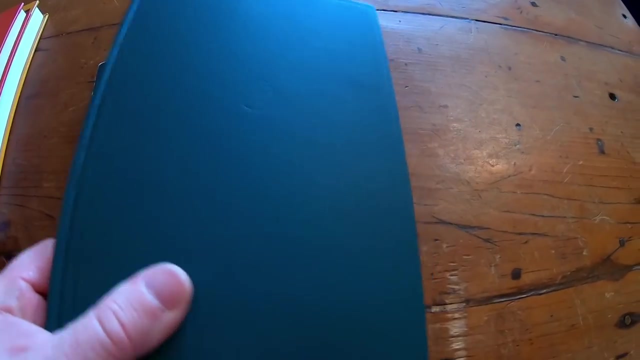 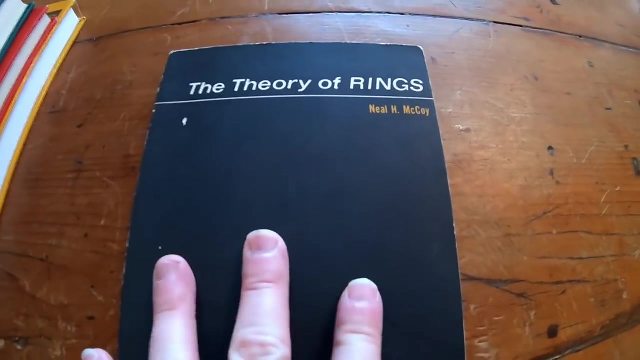 problem book here in classical ring theory. It's just got exercises in ring theory. It's a great book. But again, you have to know some math to really get into this. You have to know some abstract algebra. Here we have another abstract algebra book. This is Topics in Ring Theory by Barchet. Just another ring theory book. This one here is the one by Burns. This is another ring theory book. Again, very, very advanced stuff. You want to know abstract algebra before jumping into this. And perhaps the most famous one that you see out of this pile that I had is the one by McCoy. This is the Theory of Rings. This is considered a classic in ring theory. So 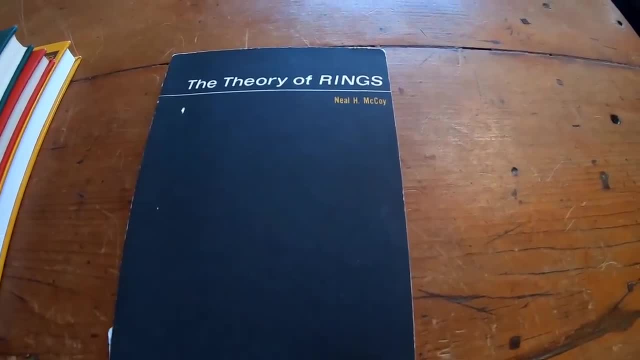 this is something you could study after you've learned some abstract algebra. So that's it. 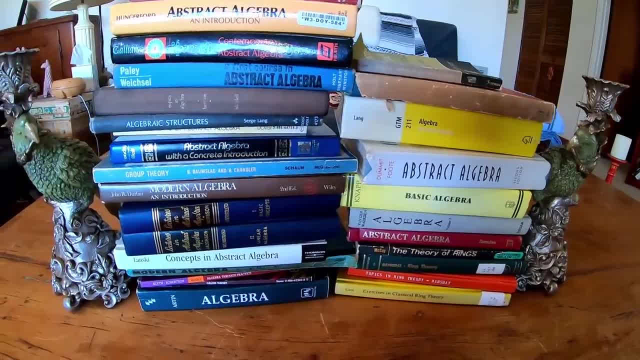 That's how you can learn abstract algebra from start to finish. And there's really no finish. 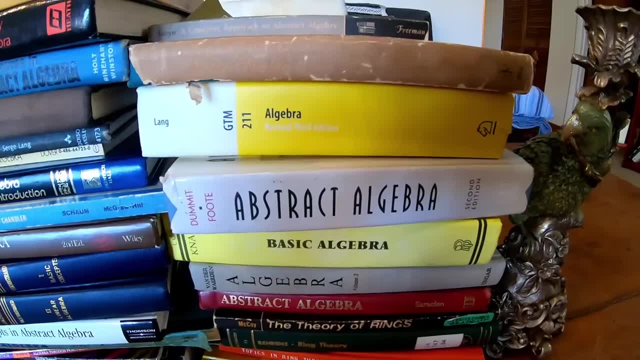 But if you get to something like Lange's Algebra and you actually learn all of the material in this book, I mean, I don't know everything in this book. That's pretty insane.